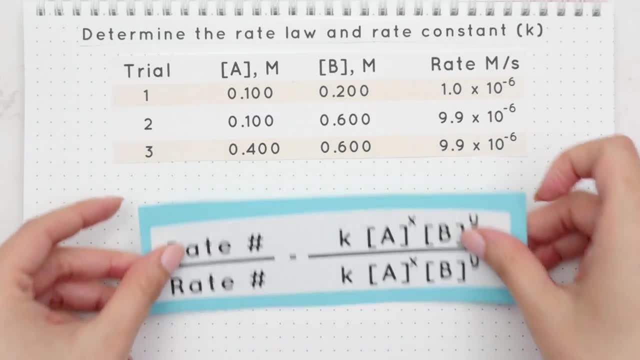 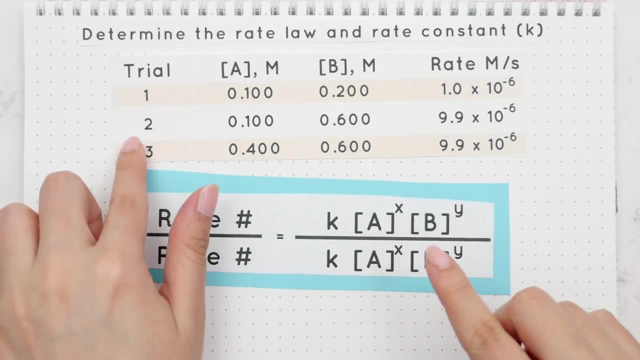 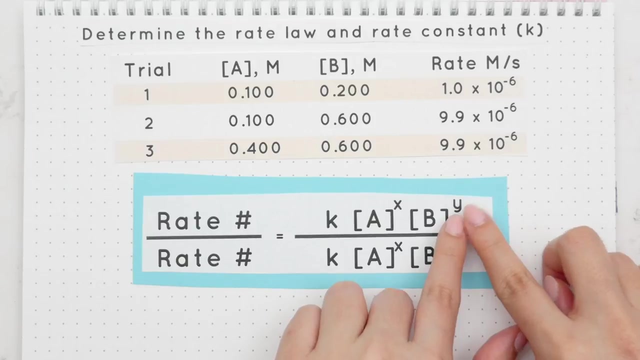 measured in molarity divided by seconds. We'll use this formula to solve for x and y, which are the reaction orders. Since there are two unknowns, we will pick trials two and one, because they have the same values, which would cancel out, and we would be left with just one unknown, which is y. 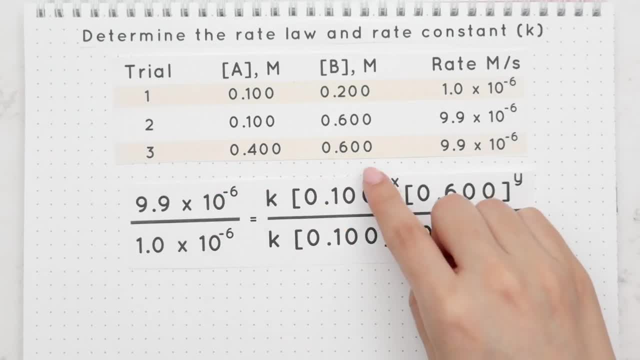 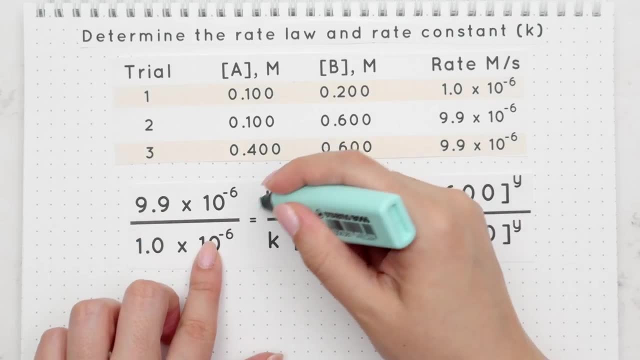 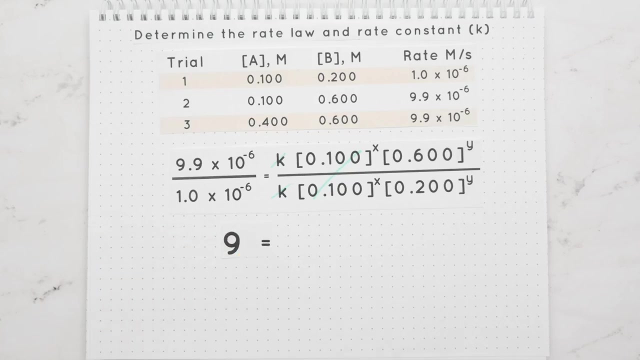 so we will divide rate two by rate one and plug in the values for reactant A and B. Next we can cancel out like terms, so the k's cancel and this entire term cancels out. When we divide the left side we get 9, and when we 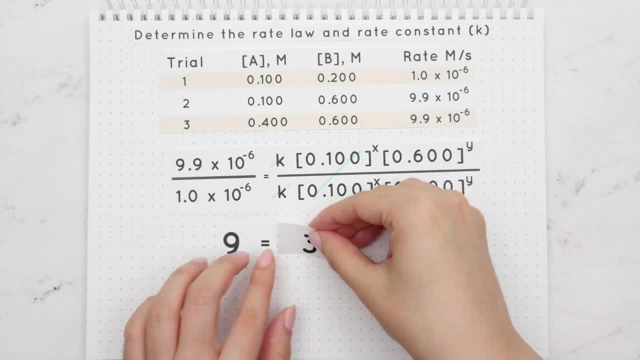 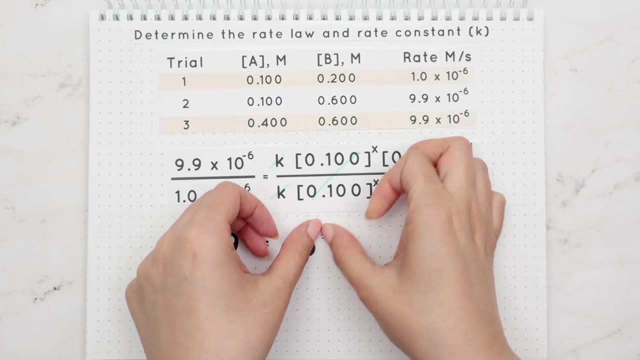 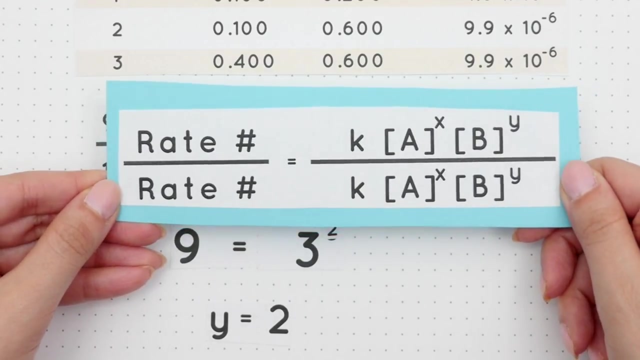 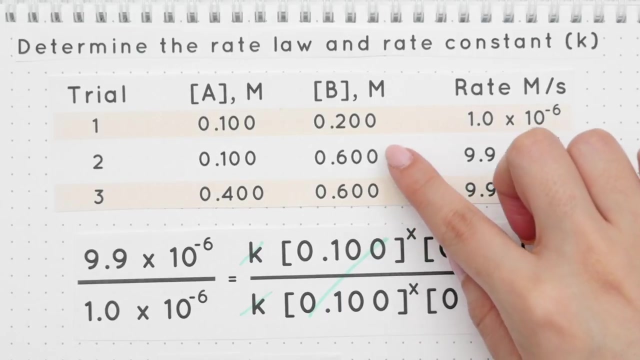 divide 0.6 by 0.2, we get 3.. That 3 still has an exponent of y, and since 3 squared is 9, then y is equal to 2.. Let's solve for X using this same exact process, but this time we will use trials 3 and 2, since reactant B does not change. 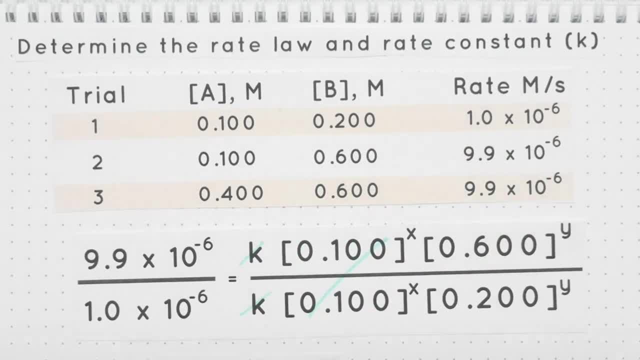 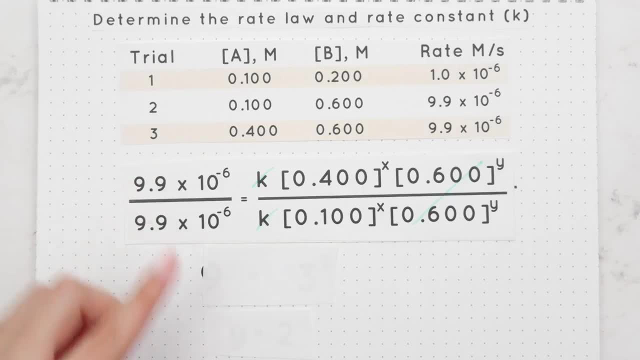 and this time that will cancel out. When we plug everything in, we get this: We can cancel the k's and the y's. and when we divide the left side, we get 1.. Dividing 0.4 by 0.1 gives. 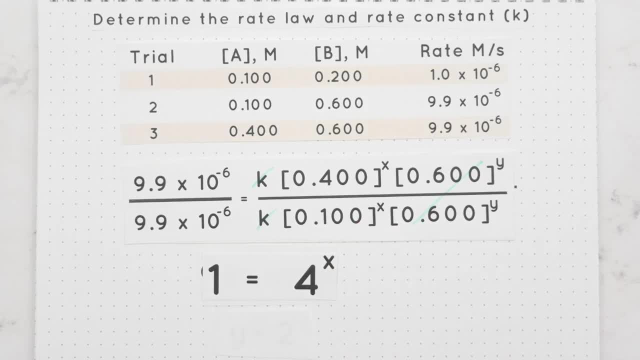 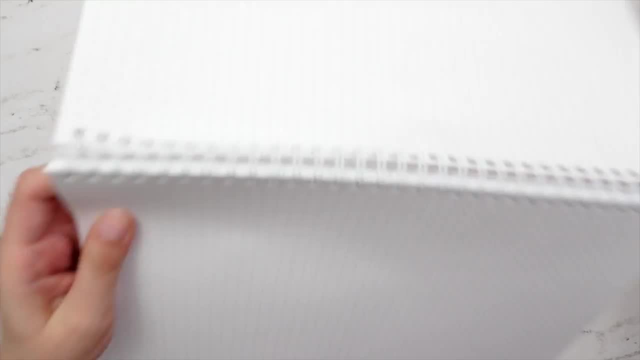 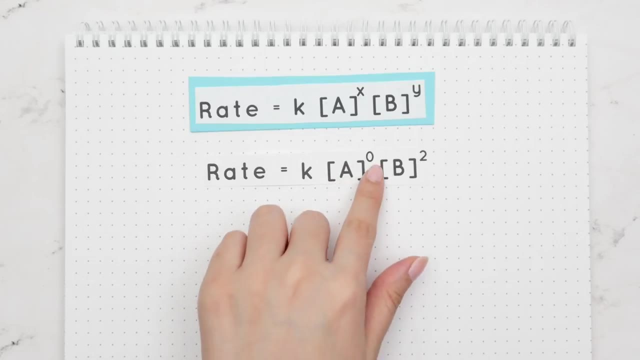 us 4 to the power of x. Now for this one, remember anything raised to the zero power is 1, so X must equal 0. Replace the X with 0 and the Y with a 2 and we will get this. but remember anything to the zero power is 1, so our actual rate law. 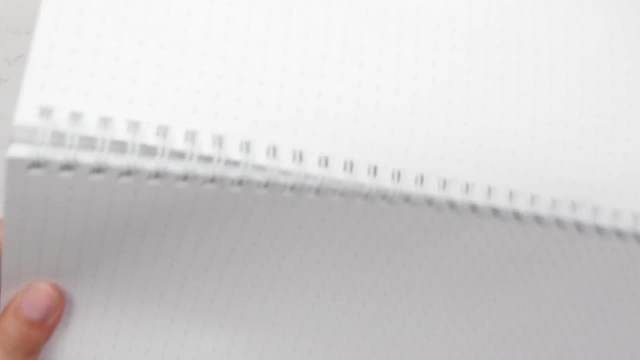 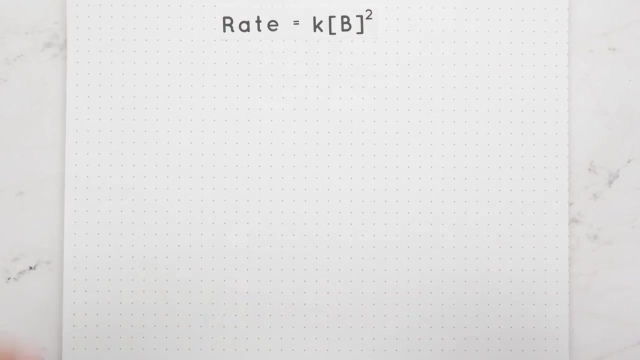 only includes reactant B. But wait, don't forget about your rate constant. We must use the rate law to find the rate constant K Using the known values in the table. we will plug that all in, Since all our numbers in the table follow some. 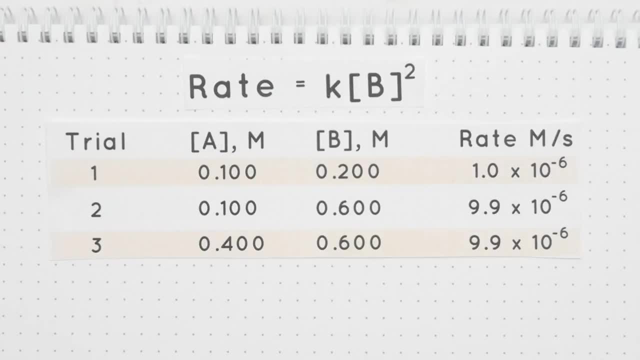 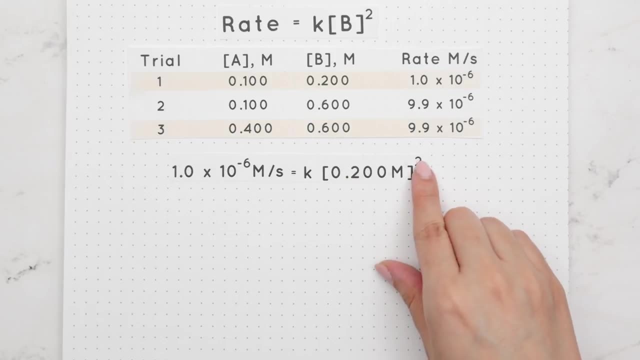 sort of pattern, then it does not matter which trial we use. In this case we will use trial 1 and plug in the values Square, the 0.2 and the unit and we will get this Divide over that 0.04 to both sides and